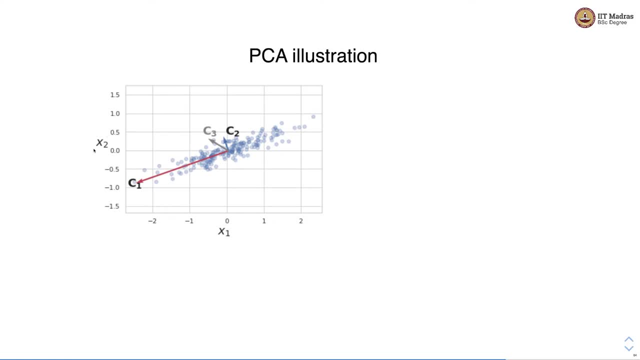 samples in the feature space bounded by x1 and x2.. Now we are trying to evaluate three vectors. for being the first principal component Now, these three vectors are c1, c2 and c3.. So what we do is we try to find out, we try to capture the variance covered by these three. 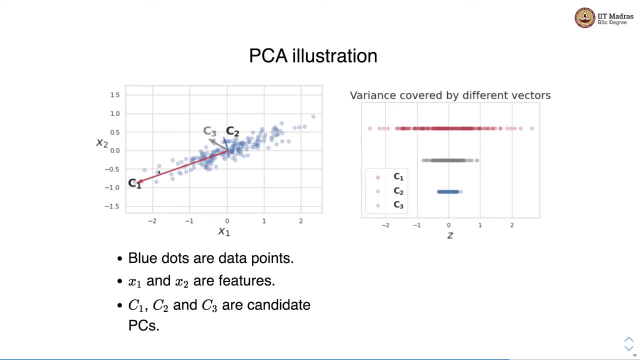 vectors. For doing that. what we do is first we project the original data point on these vectors and we find out what is the variance captured by each of the vector. So z is the projection of the original data points to the principal, to the candidate principal. 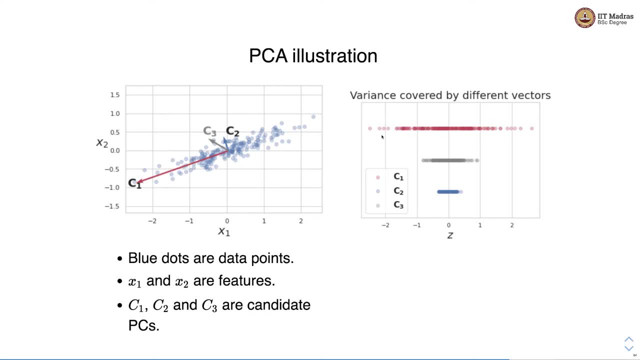 component vectors. So the red points over here is the projection of the data points on the first principal component. The grayish points are projection of of the original data points on the, on the second principal, on the third principal component, which is in gray, And then we have the, the bluish kind of projection. 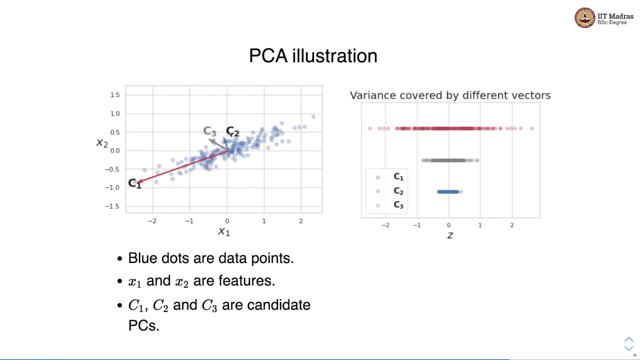 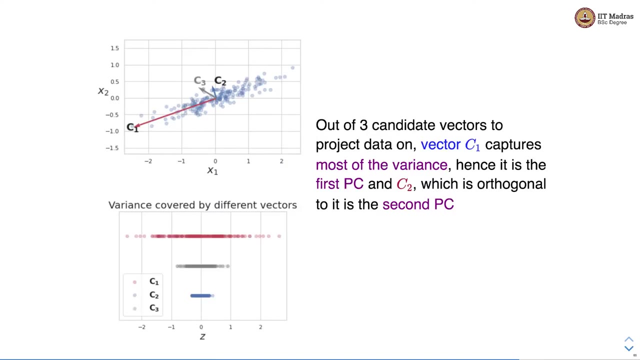 which is projection of the original data point on the vector c2.. So you can easily see that the maximum variance, or the bulk of the variance, is captured by the vector c1.. So out of these three candidate principal components, the vector c1 captures most of the 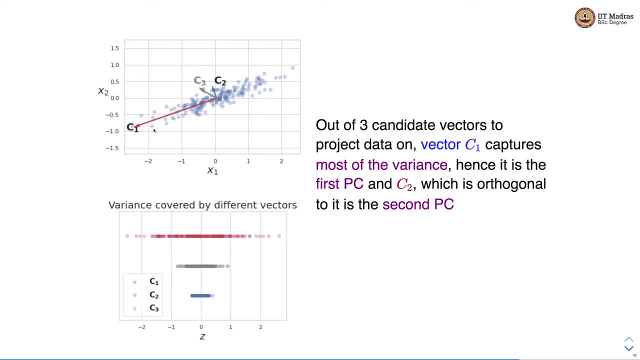 variance in the data And hence we make c1 as our first principal component. Now, even though c3 captures the the lesser variance than c1, but better than c2, we do not select c3 as the second principal component because the subsequent principal components have to be orthogonal. 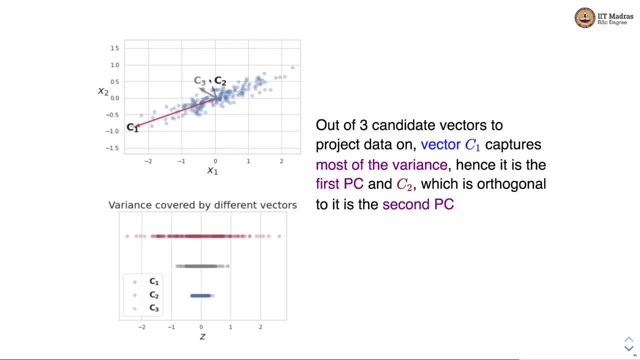 to the first principal component. Hence we select c2 as our, as our second principal component, because among different, different vectors that are orthogonal to c1, c2 captures most of the variance in the data. Hence c2 becomes our second principal component. And when we capture, when we, when we,